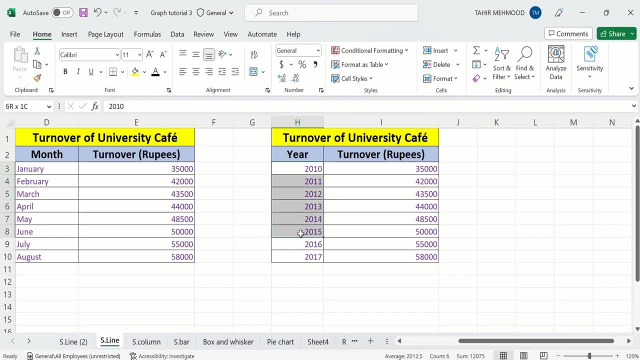 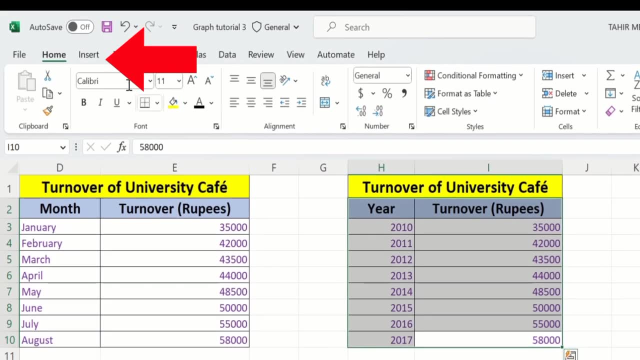 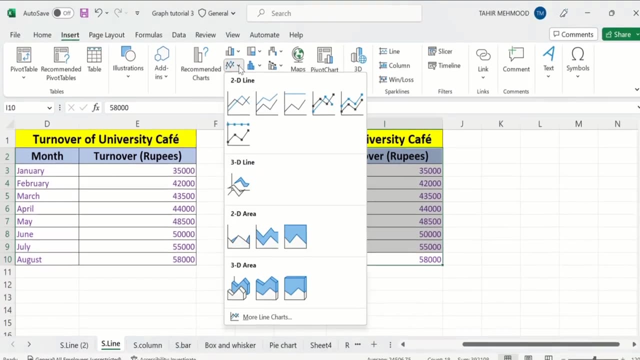 Because Excel will recognize these values as y-axis values, For example, I will select this one. Go to insert option And in insert option you will find the option of line graph- Line graph under charts. Click here and I will select this one. 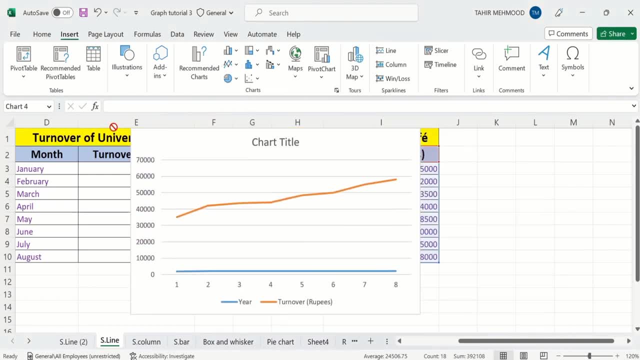 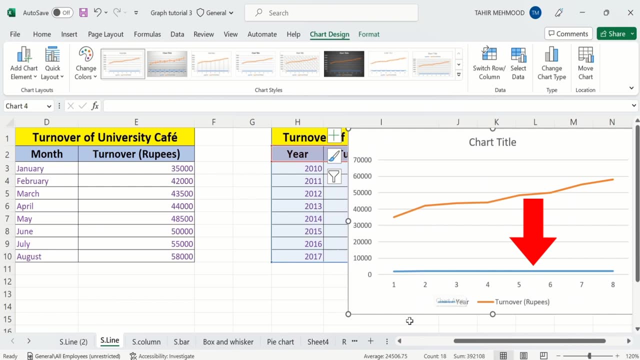 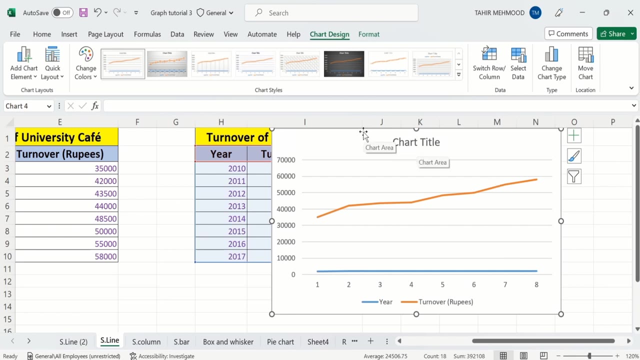 Now you can see here the x-axis values was in years, And Excel has displayed 1,, 2,, 3, 4 as x-axis values. So how can we address this issue? Firstly, I will place it here Now data is also visible to us. 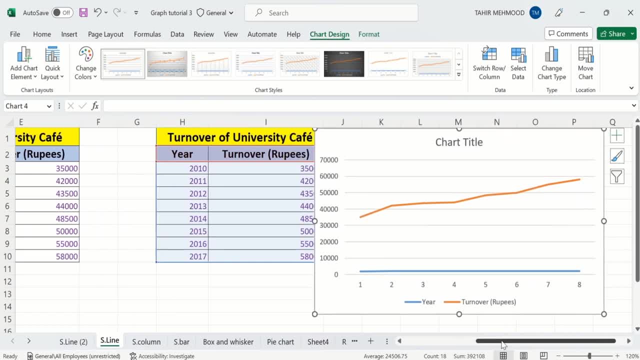 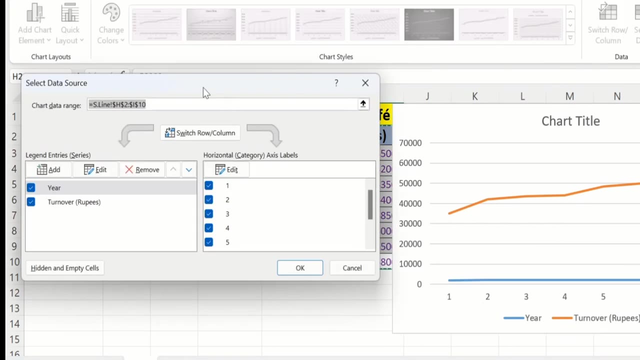 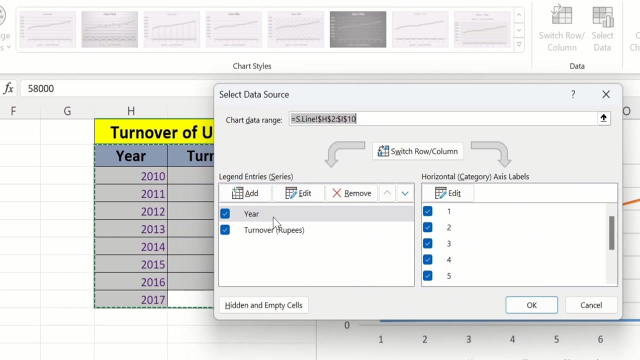 After that, select line graph, Select the x-axis. I will select this one. After selecting, right click And here you will find the option of select data. Click on it Now. here you can see. here we have two pan. This one shows the y-axis data and this one shows the x-axis data. 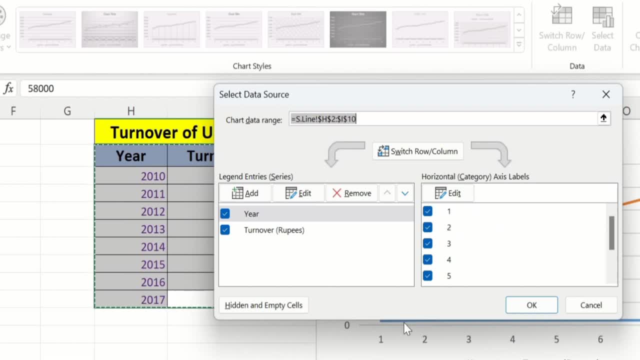 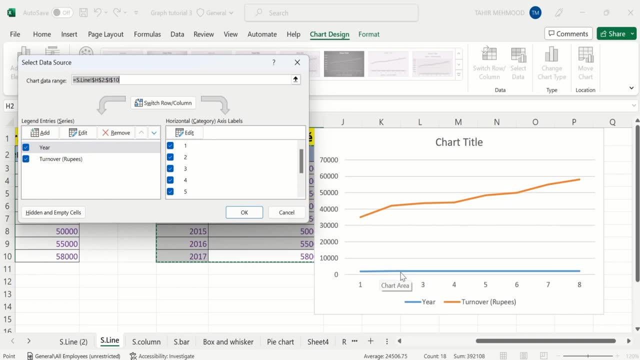 You can see here numbers are displayed here: 1,, 2, 3- and these are displayed on x-axis. Now I am interested to remove this year data series because this is the x-axis values instead of y-axis values, So firstly, I will select this one. 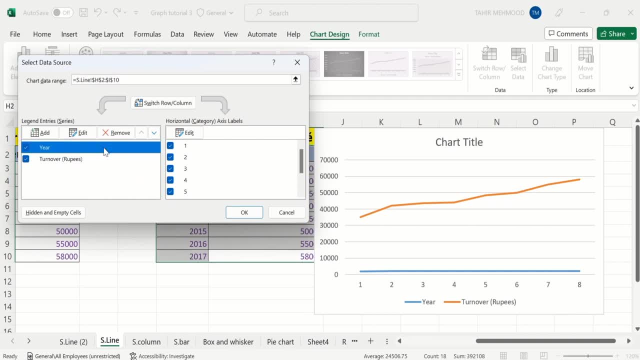 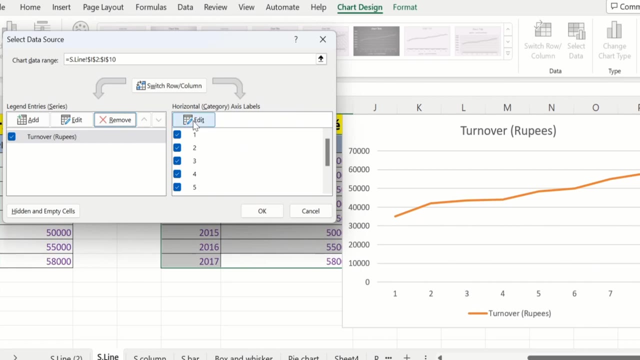 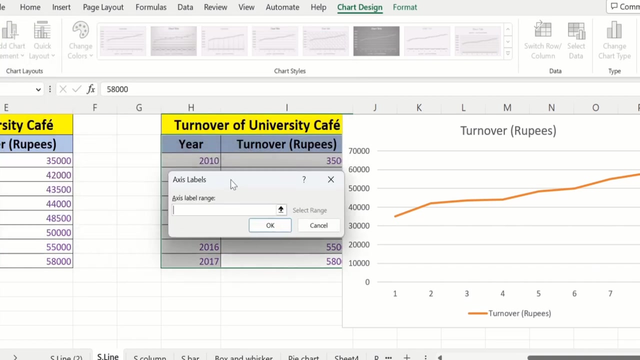 Now you can see here. I have selected year data series. After selecting, click on remove. Now you can see here: years are removed from our graph. Now our task is to replace these numbers with years. I will click on edit option- Place it here. 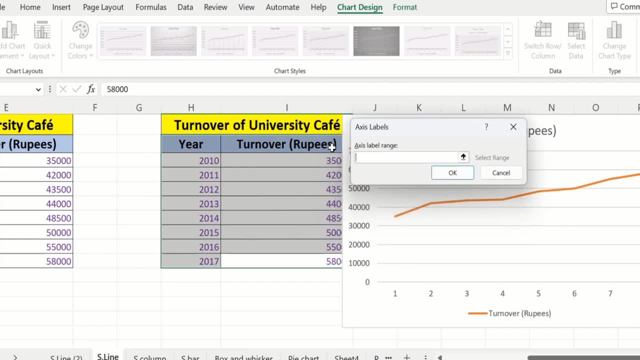 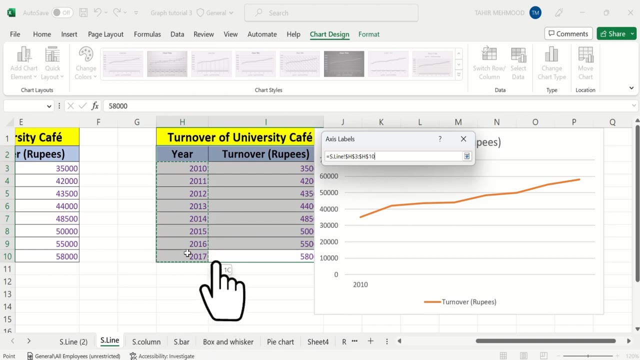 Now you can select any values. For example, I want to replace these with years. Click on here And, using dragging option, I will select remaining rows, cells, And a small box appears which shows that I have selected 8 rows and 1 column. 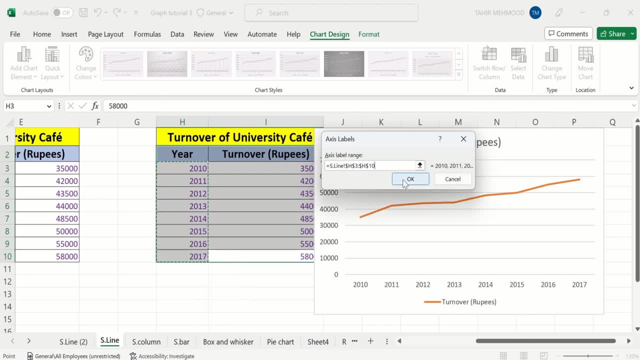 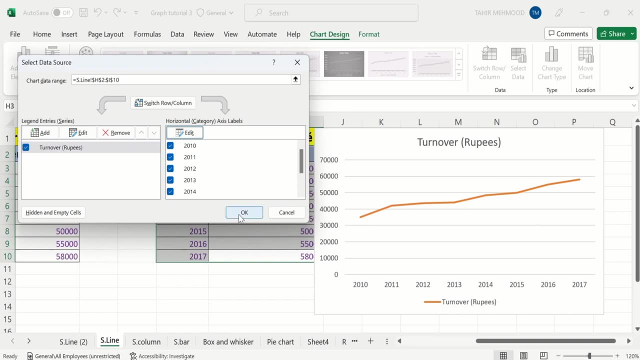 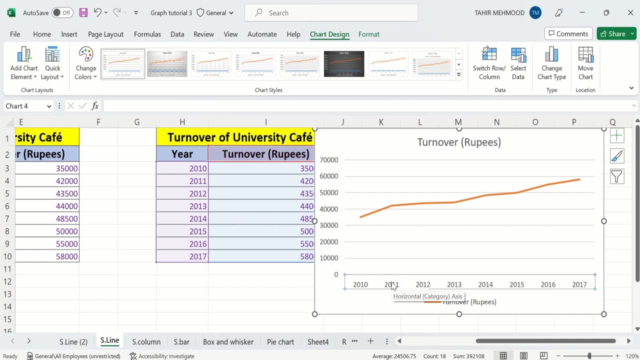 After selecting that, click on ok. And now you can see here that the numbers are replaced with years. After doing that, click on ok And you have successfully replaced the values. Similarly, if I again want to replace these values, I will simply right click.